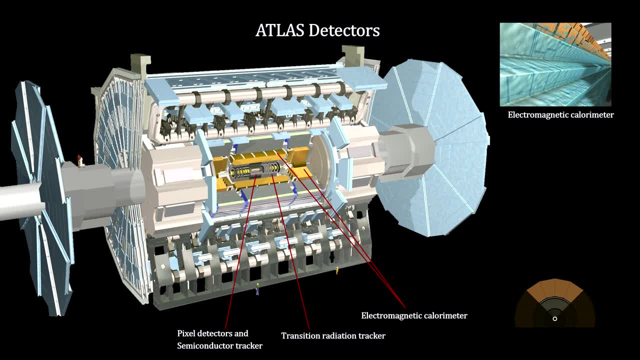 layers is liquid argon. at minus 180 degrees centigrade. Immersed in the liquid argon is a copper grid. Passing particles drive electrons to the copper grid. The particles are then passed through the copper And measuring the number gives us the energy of the particle. 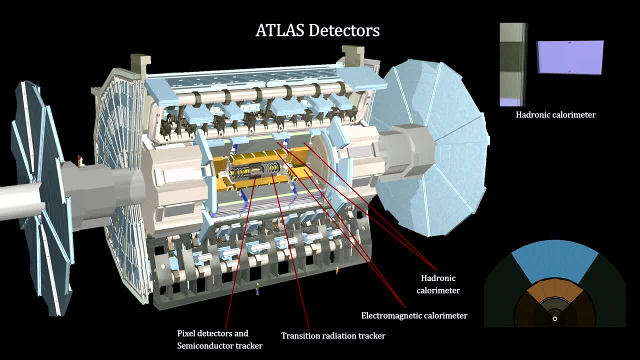 The hadronic calorimeter measures, the same for hadrons like protons, neutrons and mesons. It is a large array of steel and scintillator sheets. They create photons when struck by charged particles. Light fibers carry the light to intensity measuring devices. The light fibers are used. 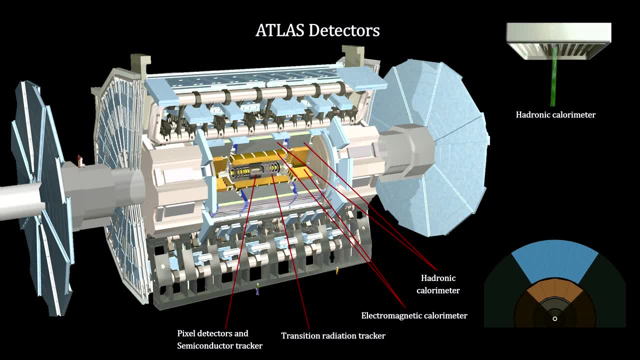 to measure the energy of the hadrons entering the calorimeter. The light intensity gives us a measure of the energy of the hadrons entering the calorimeter. At the outer layer is a muon spectrometer with a surface area the size of several football. 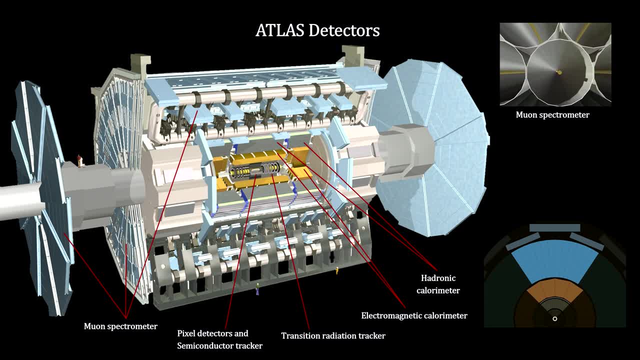 fields. In the attached chambers there are tubes also filled with gas. The electrons that are generated by the passing muon drift to the center. This enables the system to determine its track. What do you think about this? Here are a few examples. 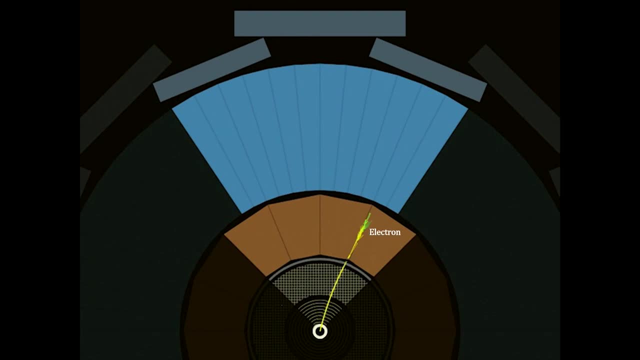 Electrons plow through the inner detector, leaving a trail before stopping in the electromagnetic calorimeter. Photons will act the same in the calorimeter, but they do not leave any track through the inner detector since they have no charge. Protons leave a track but will most likely pass through the electromagnetic calorimeter. 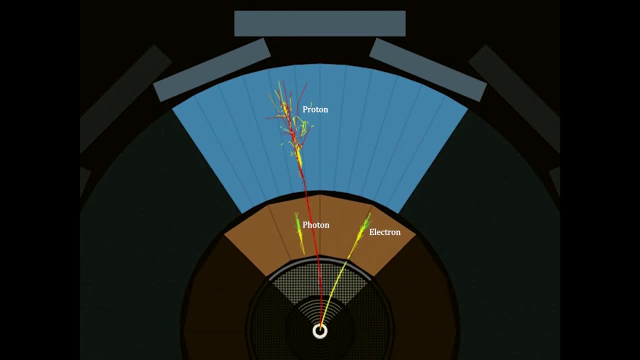 But not all protons work the same way. We will be using protons for this lesson. Let's into the hadronic calorimeter. Neutrons behave in a similar way, but leave no track through the inner detector. Muons pass all the way through ATLAS. 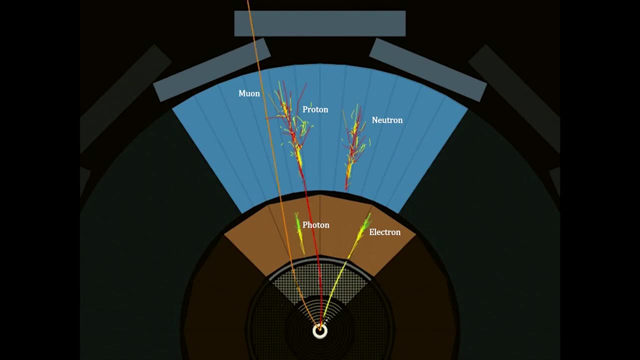 leaving tracks behind in every layer And, as was the case with beta radiation, neutrinos pass all the way through ATLAS without being detected at all.